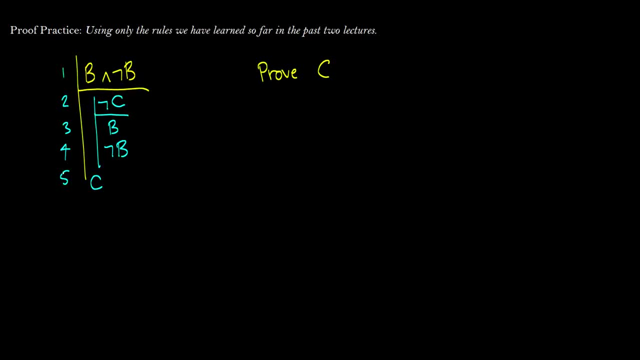 here. I'm not going to annotate every single line, but this will be AND elimination, AND elimination. This will be an assumption, And we'll get our final results using 2,, 3, and 4 with reductio ad absurdum, Because we have a contradiction of B and not B. we can. 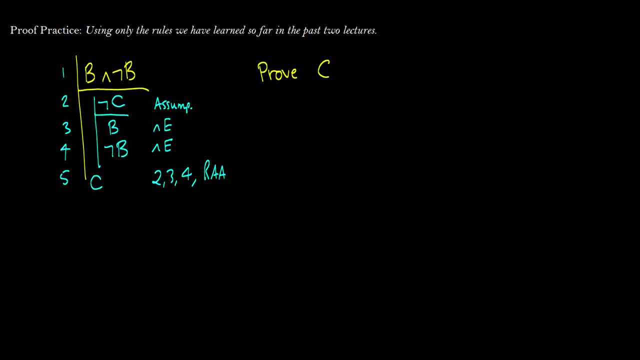 negate or take away a negation from our hypothesis in line two. So this is a pretty easy one, but for some reason, if you see B and not B and you see, oh, C, this is crazy. how do I do that? You have a structure and the interesting thing: 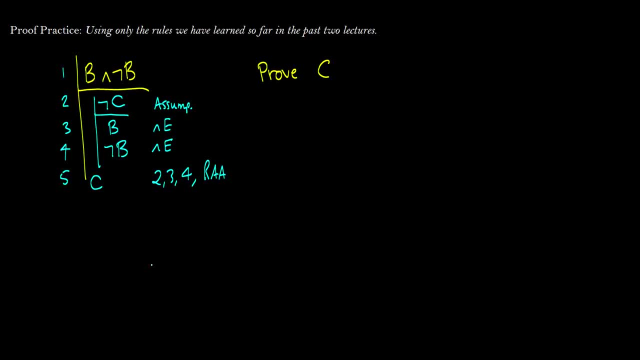 about this is that if you have two sentences- phi and not phi- you can actually prove anything you want. Literally anything can be proven with this. So this is why we do not want contradictions in our system. Alright, we want to prove from A that. So 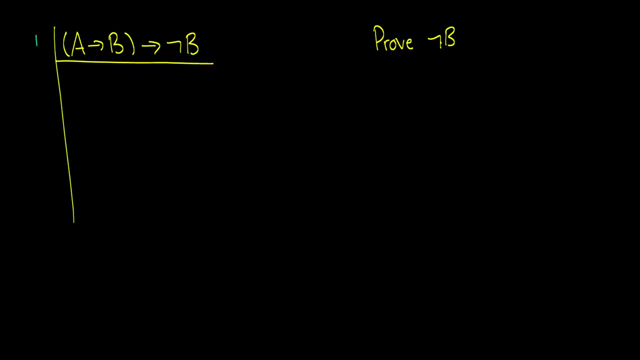 how are we going to do this? Well, we should probably figure out our end result. So our end result is gonna be B or not empty. I don't know exactly what benimarochom is called, but it should gather at least two. 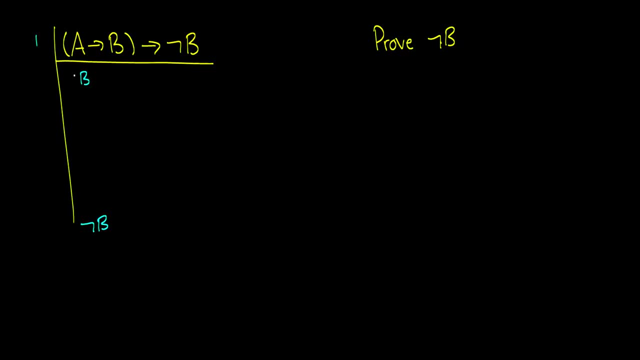 not B. so we should assume B for a contradiction eventually. so we'll open up this new sub proof and, hmm, what do we have here? well, we have a arrow B, arrow not B. and I'm gonna be completely honest here, I'm not a hundred percent sure how. 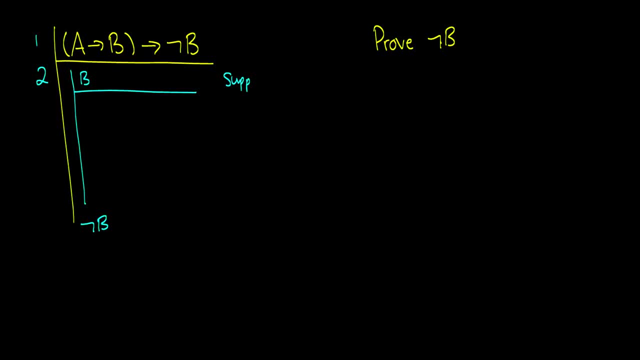 this proof is gonna go. hope we're gonna find out. let's assume: hmm, what should we assume here? why don't we assume a arrow B? but then we're gonna get not B, and then we're gonna get a contradiction of not a arrow B. so maybe this isn't. 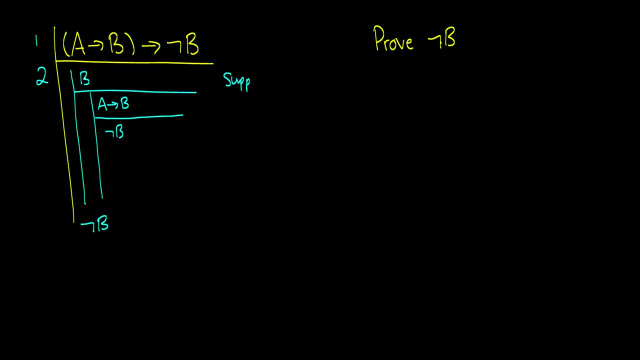 actually the way we should go, because I don't see a feasible way for me to get from B to not B, so let's do something a little bit different. why don't we assume a arrow B as a supposition and then we can get not B from this using modus ponens and hmm. 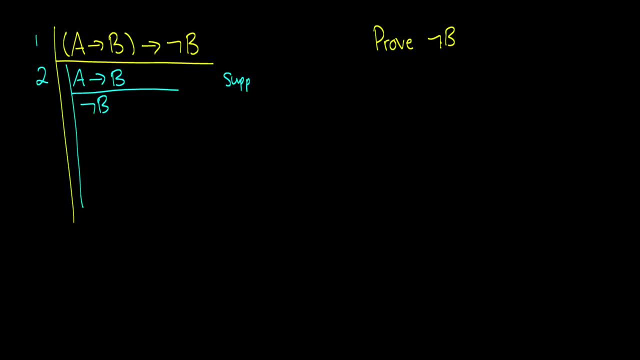 there's really nothing we can do from here either, because if we take a look, well, we could assume A, and then we could get B, and then we'd have not B reiterated, so we would get not a. but where does that go from there? I'm not sure. So when we think about what we 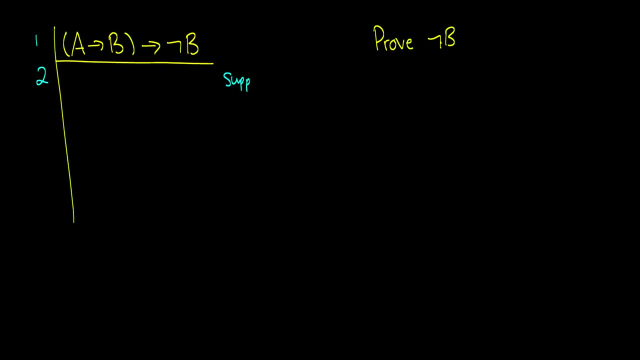 should do here? we should consider really just going with the first thing we did, which is not B, and assuming B. Now here's something you might not have seen. is that what if we just assume A on its own? And you're thinking: why would we do this? 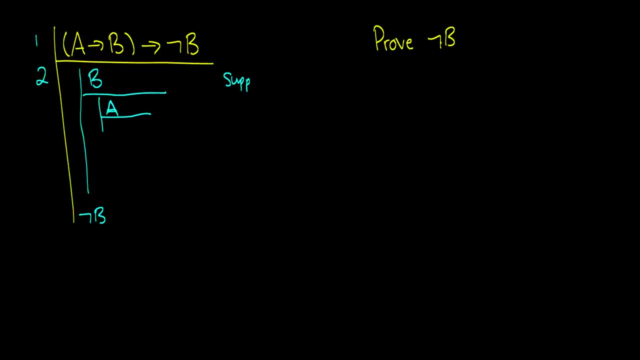 we can't get anywhere with this, but we can. we can reiterate B from line two. so we're going to suppose this and this is going to be a reiteration, and now, using a conditional proof, we are going to get A arrow B. So this is 3 to 4. 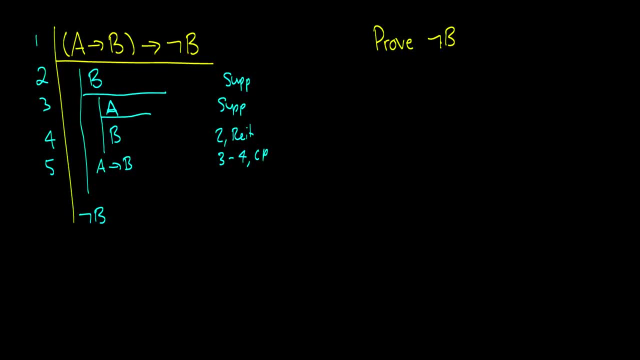 subtraction. And now, because we have a arrow b, we can get not b because of our line on 1 that says: if we have a arrow b, then we can get arrow, not b. So now, from lines 1 and 5, using modus ponens, we get not b. 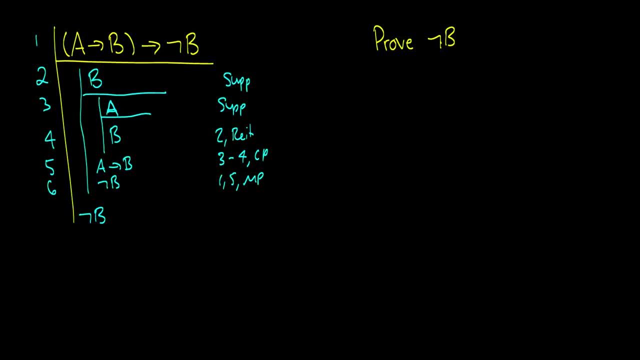 Now the interesting thing here is that we have a supposition that says b and a supposition that says not b, or a proof of not b when b is supposed. Therefore, we can use the negation of this, because we know that b cannot possibly be true. otherwise we're going to get a contradiction. 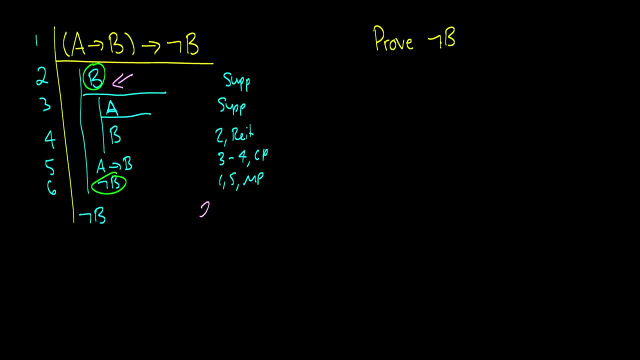 So with lines 2 through 6 and RAA We are going to get a contradiction and get not b. So I kind of took you through the thought process on this one And I really hope that when you start proofs you aren't afraid to try things. 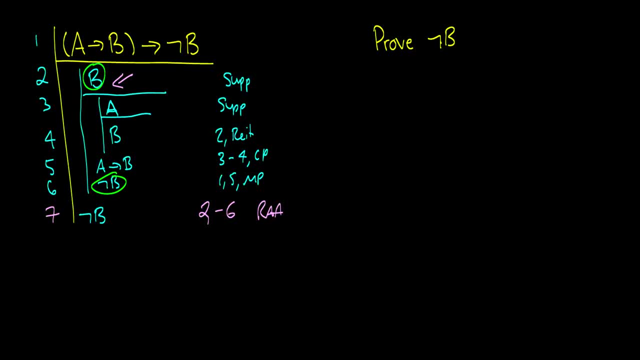 Like, I started with b and I said: let's assume a arrow b and nothing works. So I tried something different and I found out: no wait, that's not going to work at all. So let's go back to my first assumption, which was b, and see what we can do from there. 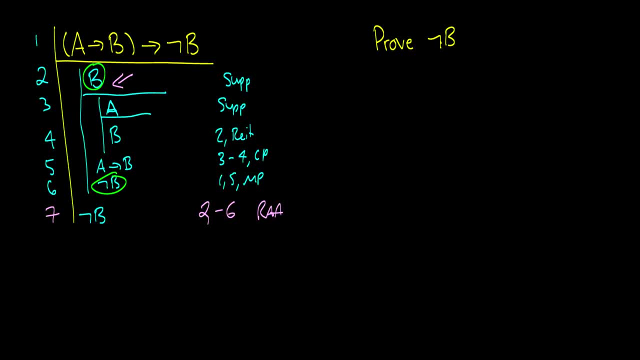 And hopefully you try that When you do these proofs. So line 3, we're going to prove not f or h from f or g arrow h and i And you have to consider the definition of or. So I will remind you that phi arrow psi is equivalent to not phi or psi. 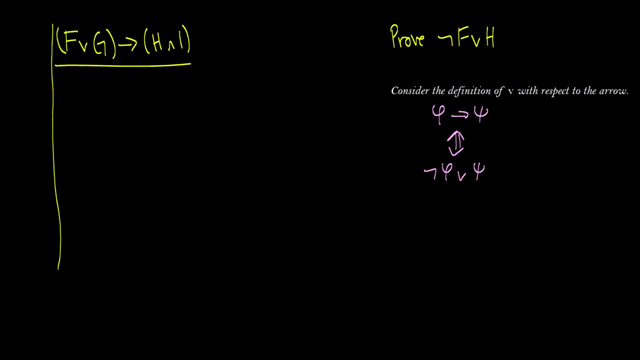 And we prove this in semantics. This is a Rule that some texts introduce later, but I don't consider definitions to be rules. In fact, in most texts, you only have an arrow in your system and you're given a definition of or from the arrow. 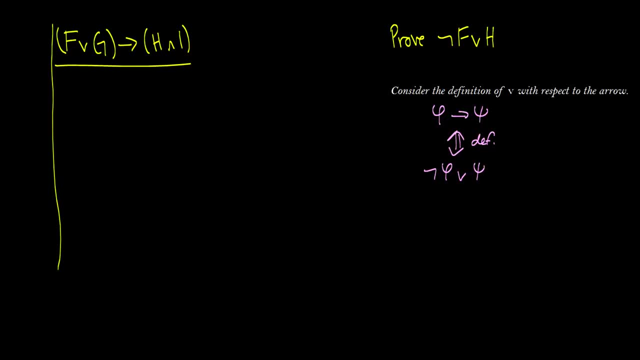 So I think it's totally acceptable just to use this as a definition in your rule. So if we have f or g, arrow h and i, Well, what should we do here? Let's assume f, And the reason we're going to need the definition of the arrow is because we're going to do a conditional proof. 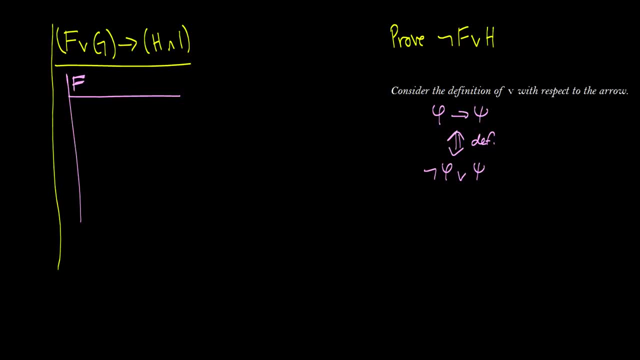 So we have an f and we want to get to h. So, if you remember, we have a rule called or introduction, So from one line we can just add or to anything we want. So we can get f or g. We can now use modus ponens to get h and i using lines 1 and 3.. 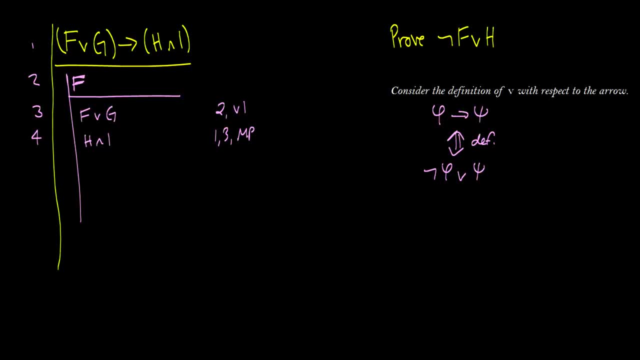 And we can then use and elimination to get h on its own, And this will be and elimination from line 4.. And now what we see here is we have a proof of f arrow h using a conditional proof. So lines 2 to 5, cp. 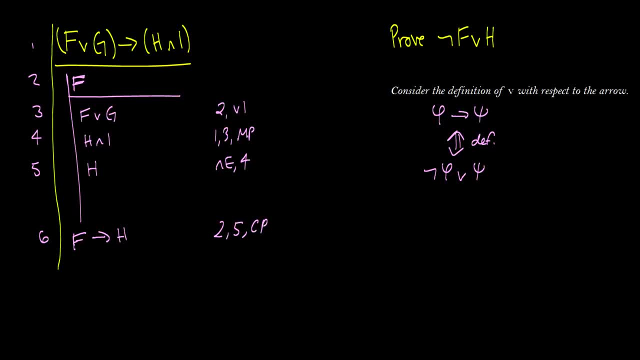 And now you say: well, what do we do now? Well, this is where this definition comes into place. And this is a tricky problem, because if you don't know this definition, you might not know that. hey, you can try conditional proof. 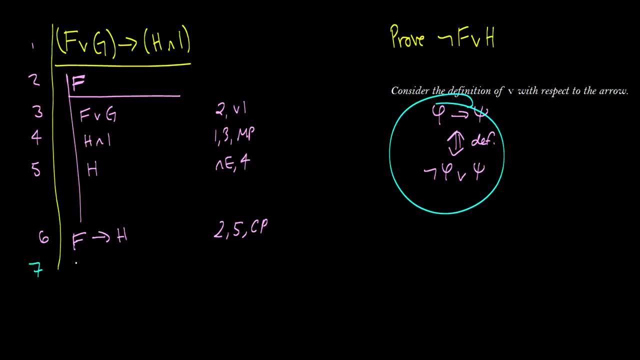 So using this definition from 7, we can say not f or h, And this would be the proof. And when we write definitions, we just write the line number and the word definition And normally you write either an arrow or an or sign one of the two. 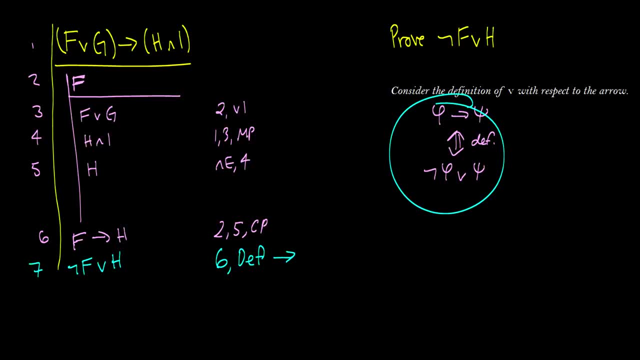 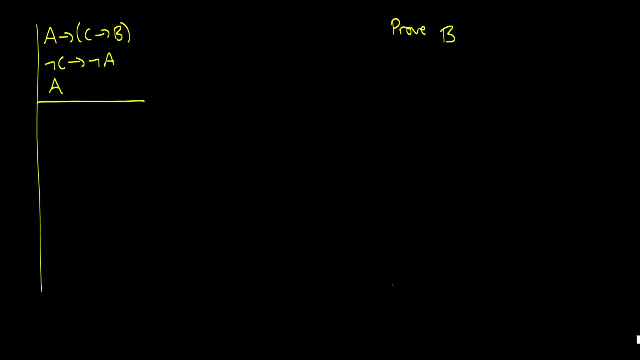 It's usually implicitly. It's usually known, if you give a line number and say definition, what you're talking about. So we have one more proof And we have a arrow, c, arrow, b not c, arrow not a and a. 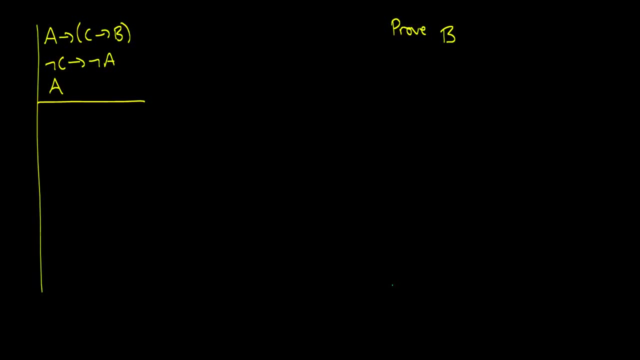 And we need to prove b. So what we see here is that we need an a and we need a c And then we can get b. So let's try for that. We already have an a, So using lines, Lines 1 and 3, we can actually just get c arrow b right off the bat using modus ponens. 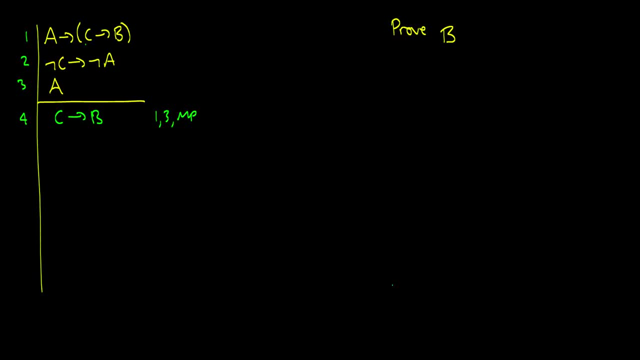 So now all we need is a, c. So how do we get a, c- Let's assume not c- for r, a, a? We're going to get a contradiction here, hopefully. So this is a supposition: With not c, we can get, not a. 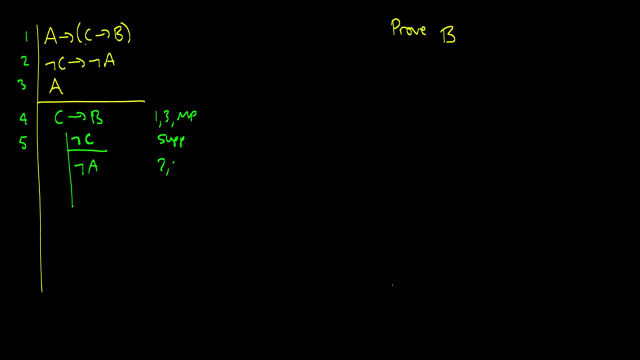 And this is with lines 2 and 4.. 5, using modus ponens, And now that we have not a, let's reiterate c back in Or reiterate a into line 7.. So this is a reiteration of line 3.. 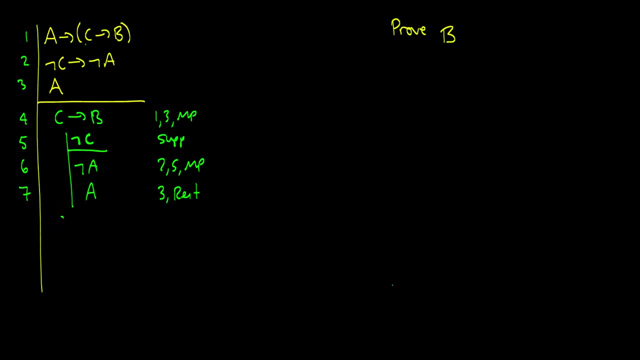 And now we see a contradiction. So with this contradiction we can just take the negation off and put c there. So this is 5,, 6 through 7, r, a, a And now that we have c, with line 9,. 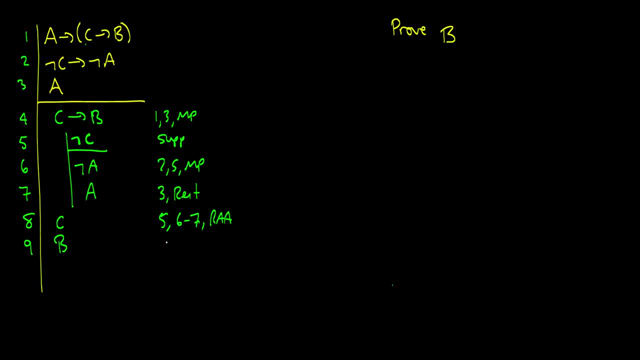 we can go to b using 4 and 8 with modus ponens, And now we have proven b. So those were some proofs. Of course, you still have to do more. You're not going to be able to finish your exams and do really well without practice.